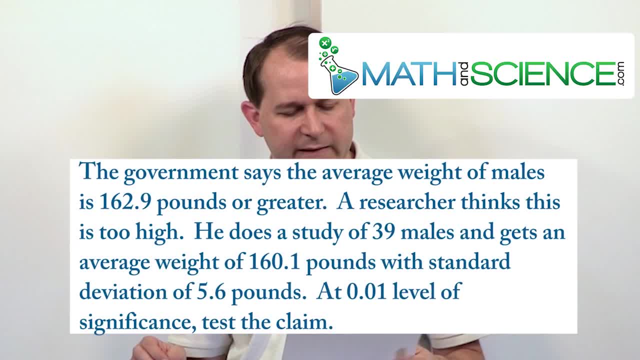 All right, so we have. the government says that the average weight of adult males is 162.9 pounds or greater. Presumably that comes from a study somewhere. A researcher thinks that this is too large. He does a study of 39 males and he gets an average weight of 160.1 pounds from his data. 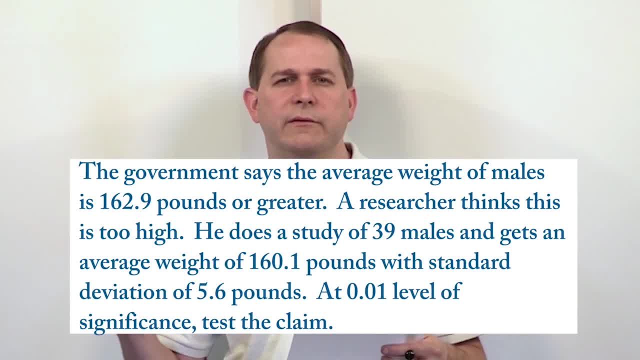 with a standard deviation of 5.6 pounds At the 0.01 level of significance test. this claim So clearly this is about the average weight of adult males. Clearly, all the weights are going to be different, right, But we're looking for the average number of the males in the population. 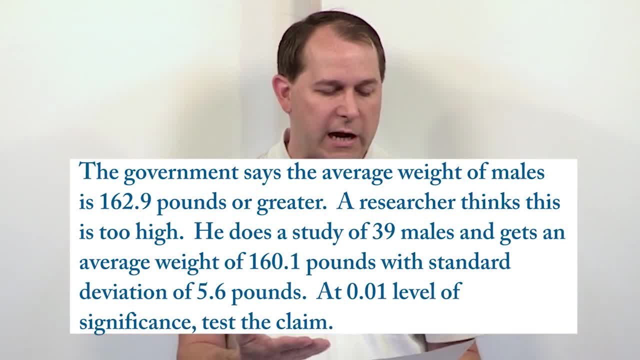 We can't test everybody. so what we do is we take a subsample, 39 in this case. We get some data from that and then we want to see if the information we get is statistically significant enough to allow us to reject the null hypothesis or not. So the first step is: let's write down the null. 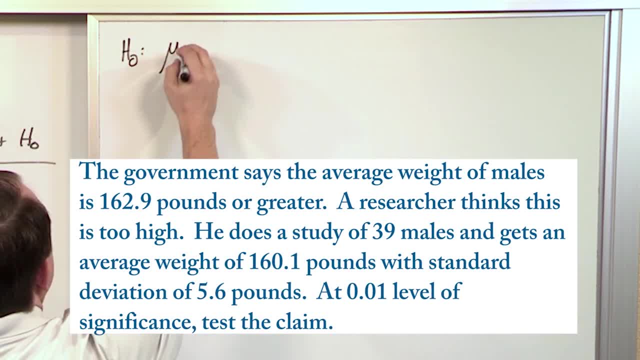 hypothesis, It is a mean, the average weight right, And the government says that it's greater than or equal to 162.9 pounds, And so therefore the alternate must be the opposite of this: less than 162.9 pounds, So greater than or equal to this. 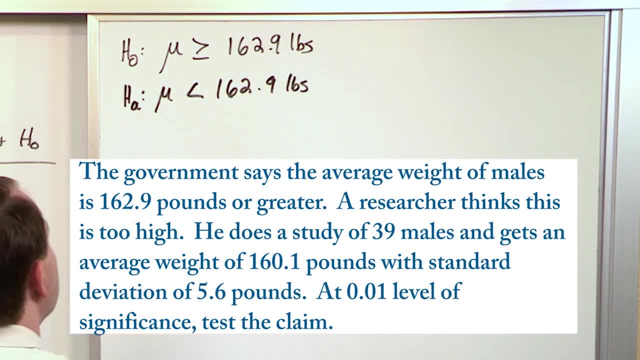 less than or that. These are opposites of one another. All right, so what does the researcher do? He thinks that this number was too big. That's why we have a left-hand arrow like this, So he grabs as many people as he can. He's not very. 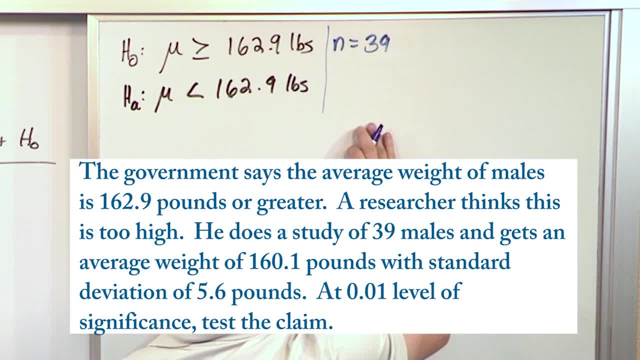 hard worker. He can only get 39 people to weigh themselves And they get an average value of these people of 160.1 pounds and a sample standard deviation of 5.6 pounds. All right, so clearly you can see that you might think that it's already going to be lining up with this. We're saying his. 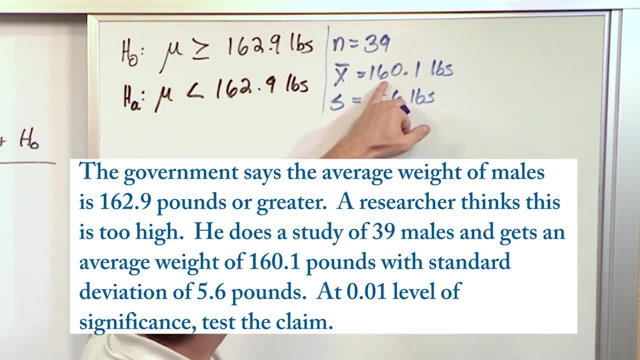 research hypothesis is less than 162.9, and that's certainly what he got, so he's pretty happy. But then he can go to the next step, and that's what we're going to do. So we're going to go to the next step, and that's what we're going to do. 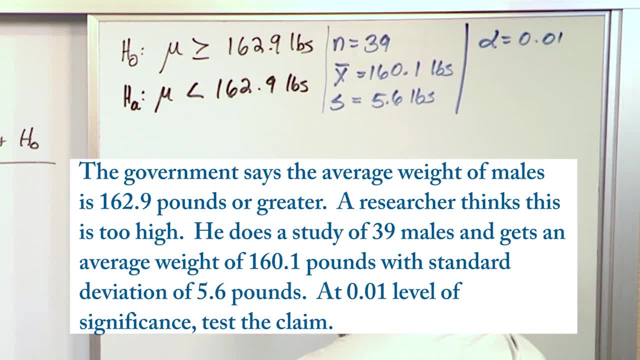 over here and says we're testing at a level of significant 0.01.. All right from this, you should know right away that the level of confidence is 0.99.. These have to add up to one, So this is basically a 99% level of confidence sort of deal. Also because the arrow points to the left. this 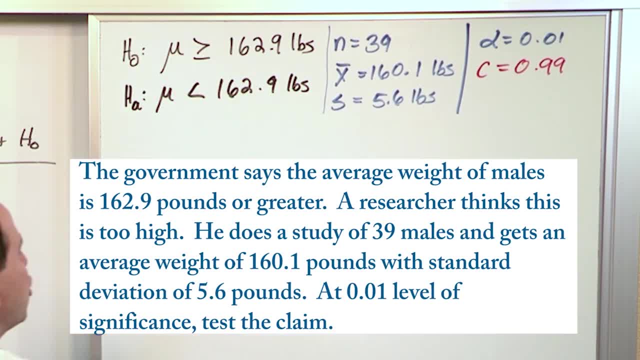 is going to be a left-tail test And we're going to be using a normal distribution because he was managed, he was able to get more than 30 samples, So we don't have to use the t-distribution or degrees of freedom or anything like that. So we're going to be using a normal distribution, So we don't. 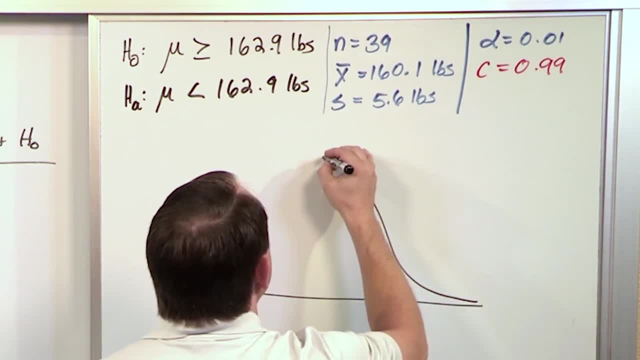 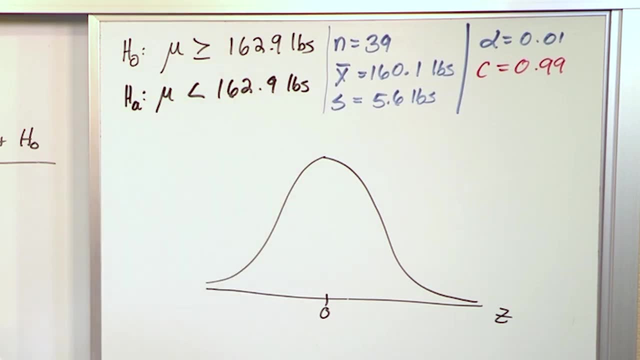 have to use the t-distribution or degrees of freedom or anything like that. So here we're going to draw a little sketch of our distribution. It's a normal distribution. It's always centered about 0, and it's a left-tail test. All right, so this data is collected. We don't know what the test. 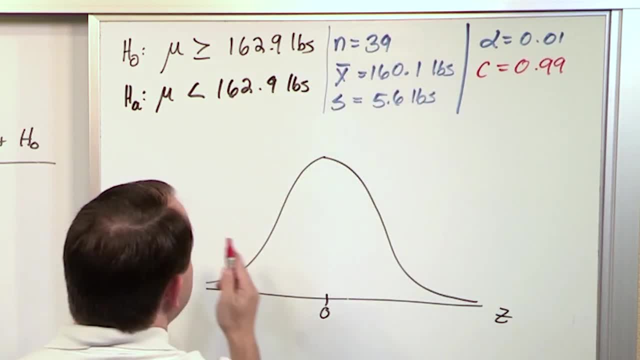 statistic is, but we suspect and hope that, since it's a left-tail test, that test statistic is going to be over here somewhere And it's going to yield a shaded region which will be more extreme than the data that we collected in this direction, since it's left-tail And we're thinking. 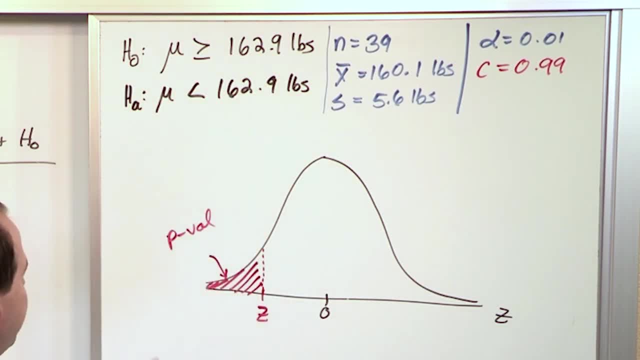 that this is going to be the p-value. That's what we're seeking, because once we have the p-value, we just compare it to the level of significance 0.01, we get our answer. So, in order to do that, 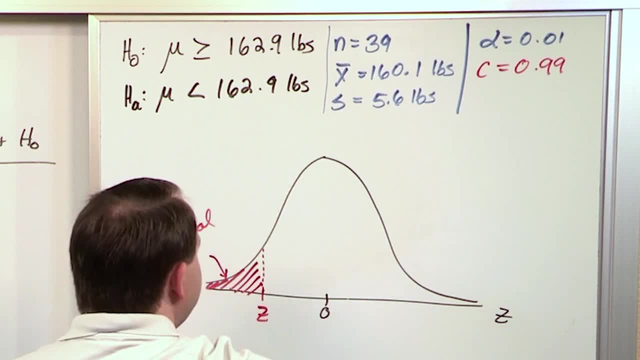 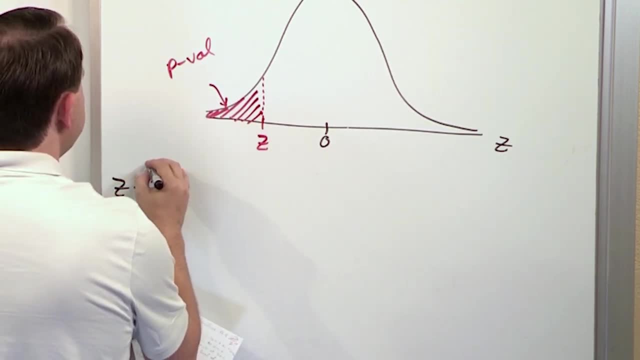 we have to find the test statistic That comes from our data. The test statistic is going to be z and it's just simply going to be the mean value of the data we collected, minus the mean value of what the null hypothesis says over the sample standard deviation. square root of n: the number of 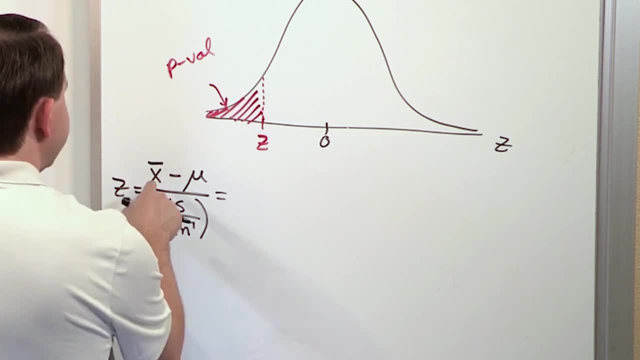 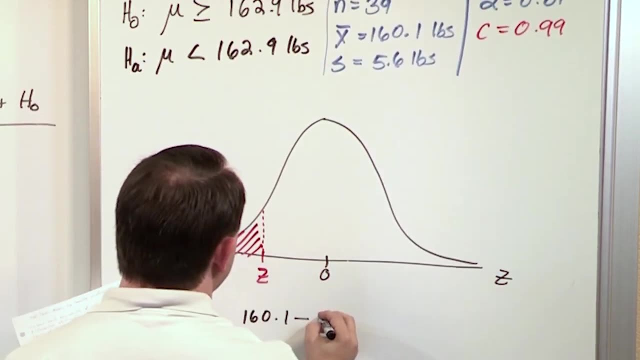 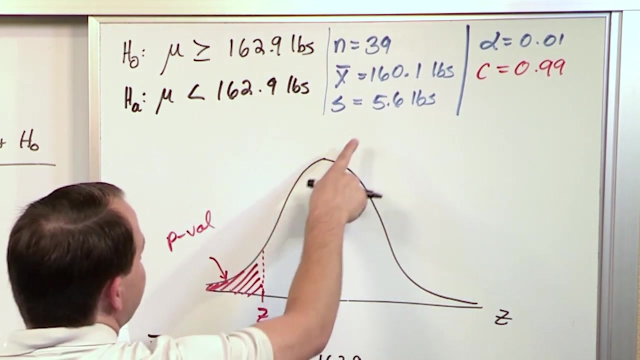 samples, And so we say this is going to be 160.1.. This comes from the null hypothesis 162.9.. On the bottom s is the standard deviation of the samples that we collected. 5.6 pounds was the standard deviation of the raw data that we collected from people. And then we have the square. 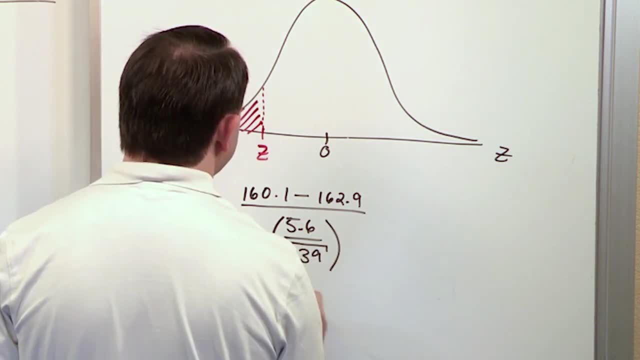 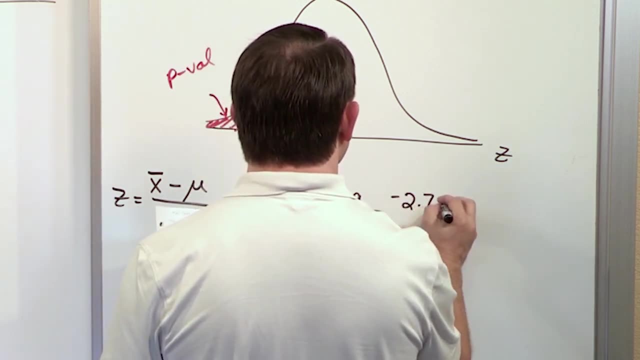 root of n, which is 39. So on the top, 160.1.. So we get 1 minus 162.9.. We get negative 2.79 on the top And on the bottom we'll leave the 5.6 for. 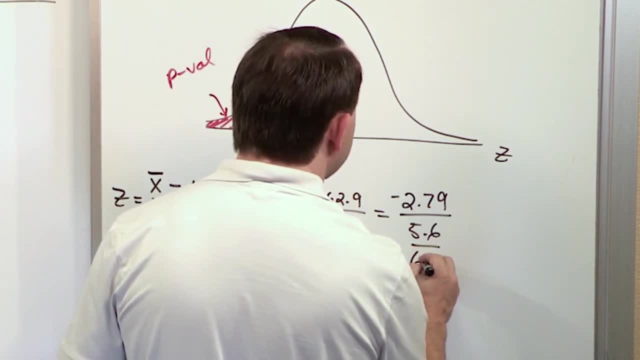 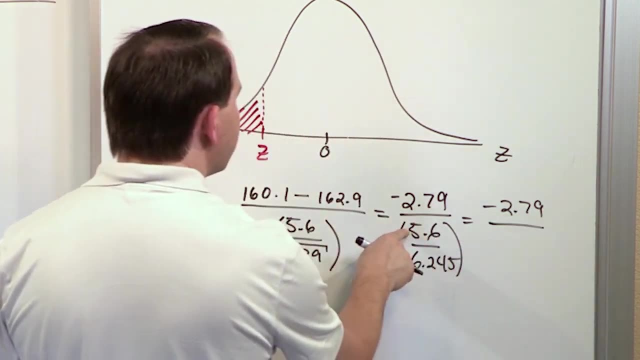 now The square root of 39 is 6.245, and we'll wrap that in parentheses, So we have negative 2.79.. And on the bottom, when you divide these numbers- 5.6 divided by 6.245, you get 0.897.. So basically, 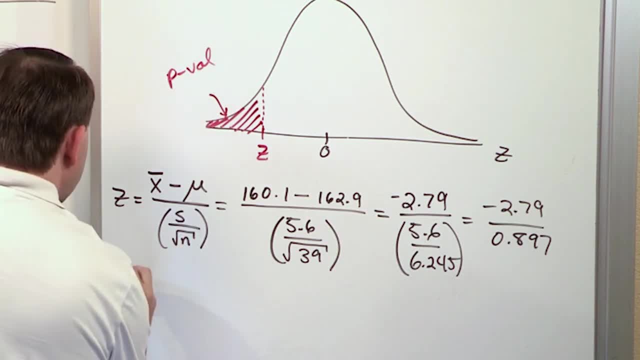 we just have to divide those two numbers And when we do that we will get a value. if z, we take negative 2.79, divided by 0.897, we get negative 3.110.. So that's good, right, Because. 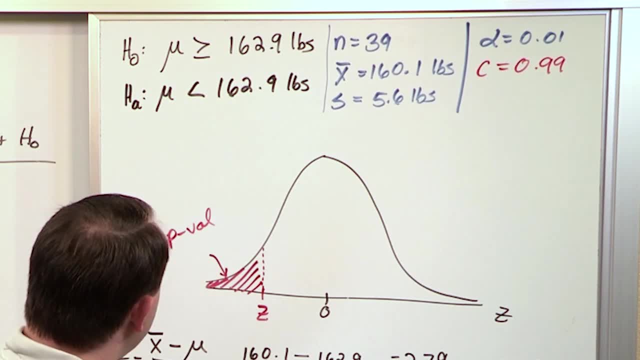 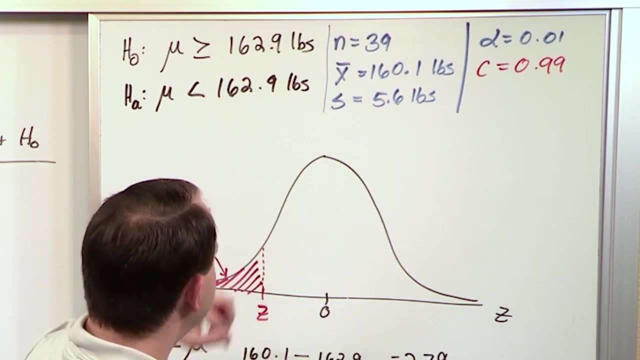 we move to the left. This is a left-tailed test. We're hoping that our data is going to pull us to the left, and it is because the average value that we got from our data was less than the 162.9.. 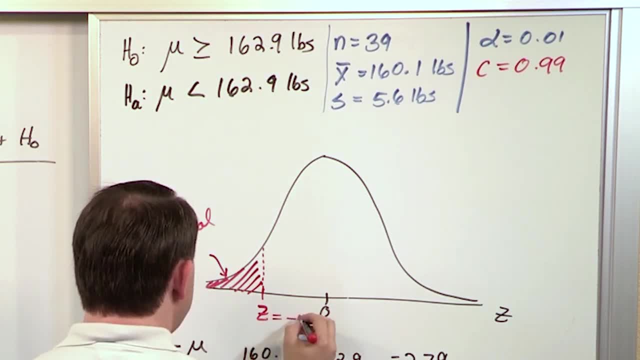 So this value of z we can now put as a value on the chart, negative 3.110.. And the question is: what is the p-value? The p-value is associated with the data that we collected. It's a one-tailed test to the left. We want the. 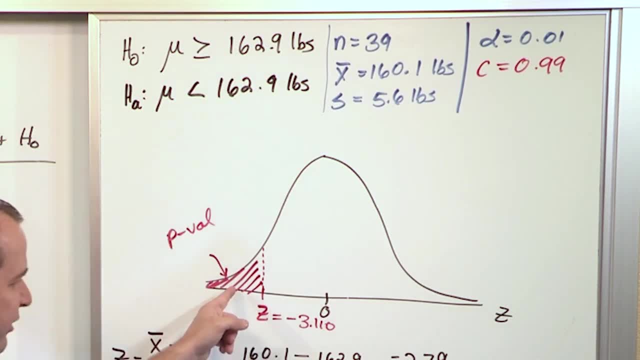 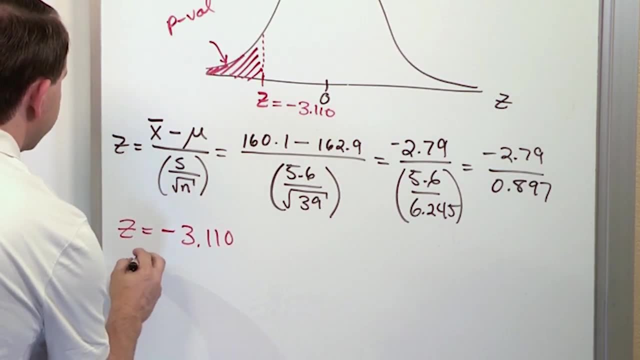 probability of samples being more extreme than what we've collected, which is the shaded region to the left of z. So you get this straight: from a normal distribution, The probability of getting z's less than negative 3.110.. The chart always returns areas to the left, so we just look at negative 3.110. 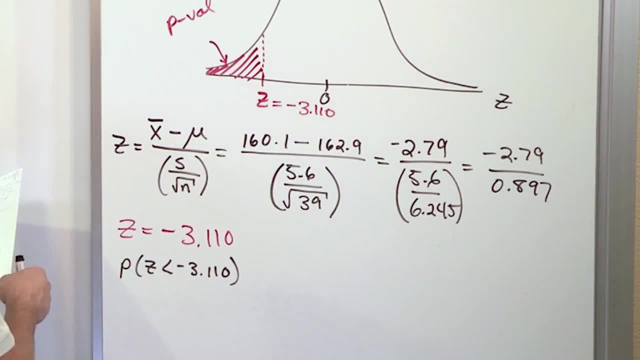 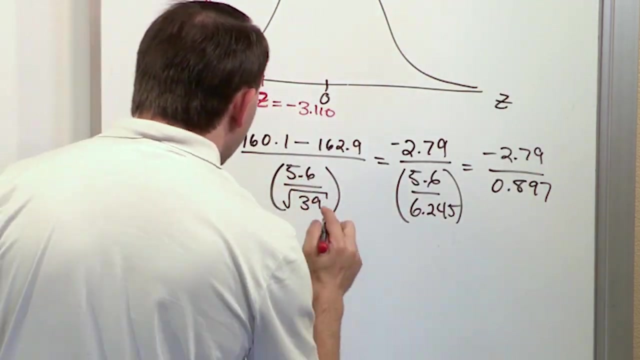 in a chart of z of the normal distribution And you're going to get a really small number, 0.0009.. So the p-value is 0.0009.. And what we do is we compare this to the level of significance for our problem: 99% level of confidence: 0.01 level. 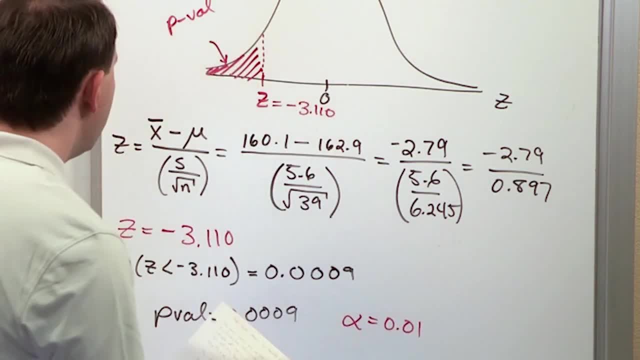 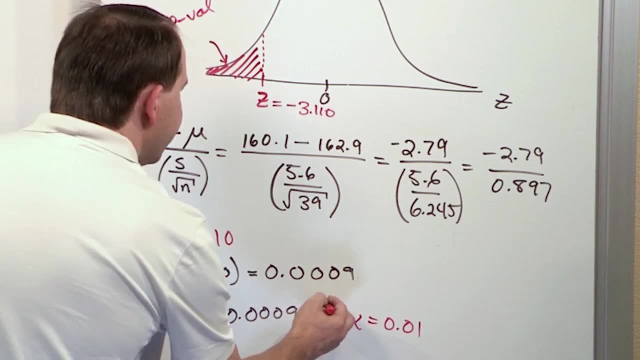 of significance. Level of significance. Which way does the arrow point Which one of these numbers is smaller? Well, this one has more zeros. So the decimal point before the number: this guy is smaller. So what we conclude is that p is less. 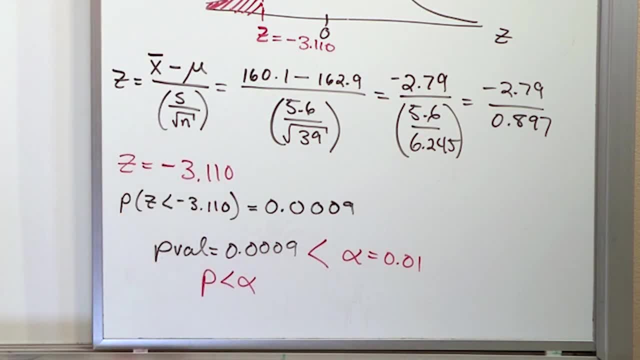 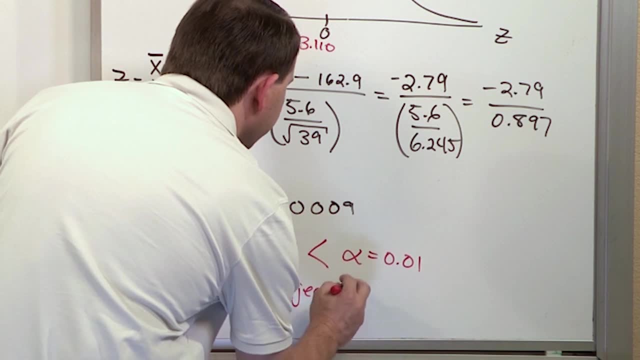 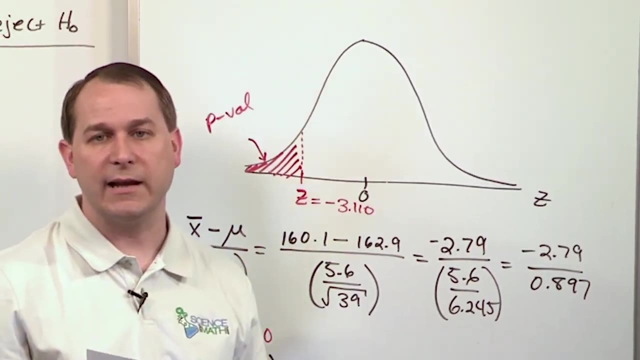 than alpha. p is less than alpha. We come over here: p is less than alpha. We reject the null hypothesis. So we say: reject the null hypothesis at this level of significance of course. So the evidence is strong, at a 99% level of confidence. to say that, because we can reject this, to say that the average 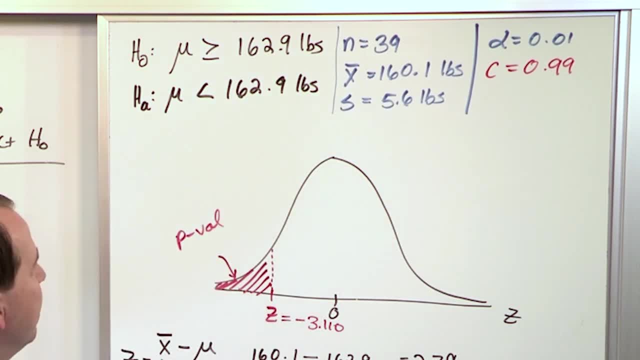 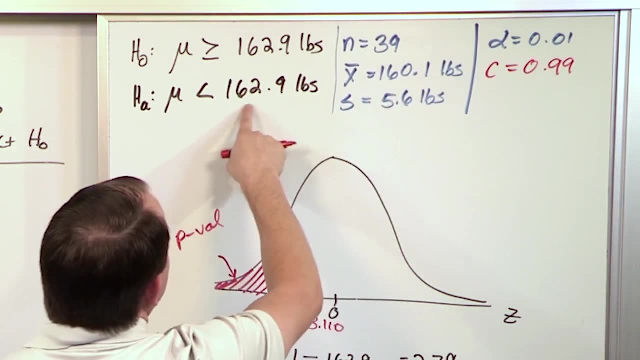 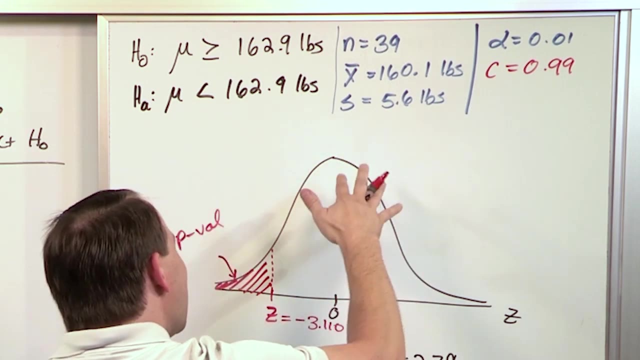 weight of males is actually less than 162.9 pounds And I think the reason that that probably came about was mostly because this value- 160.1, is pretty far is significant- substantially lower than that. You have a reasonable number of samples. Standard deviation is not too high, not. 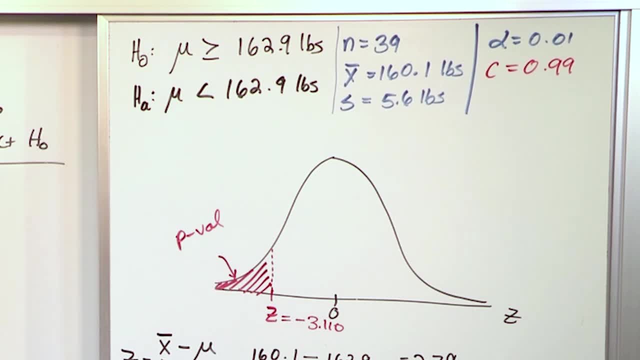 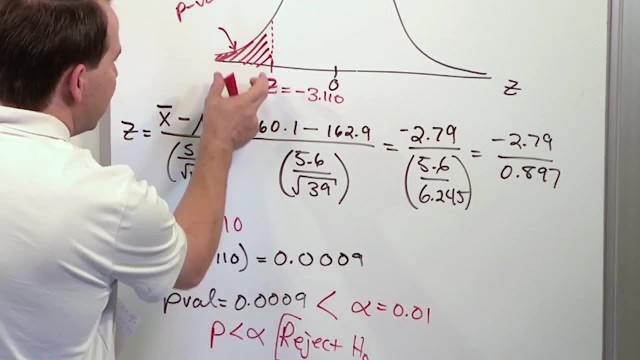 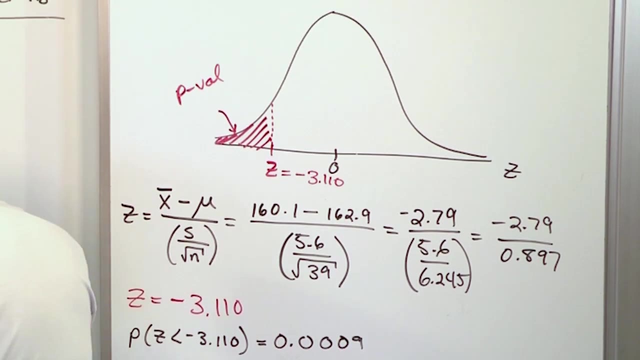 too low, So it was enough to go ahead and reject the null hypothesis. Now, if you wanted to visualize it in terms of rejection regions, what we found here is that the area here for the p-value this is less than 0.01.. So that means that if I were to plot on the same plot or on the same chart, the 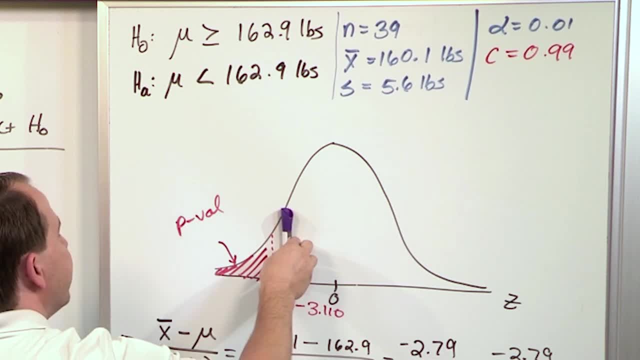 level of significance, which would be the area that we've been using for the rejection regions. it would be over here somewhere. Basically, we're saying the level of significance area is greater, So that means that that shaded region would be something like this, And then the value of z that came. 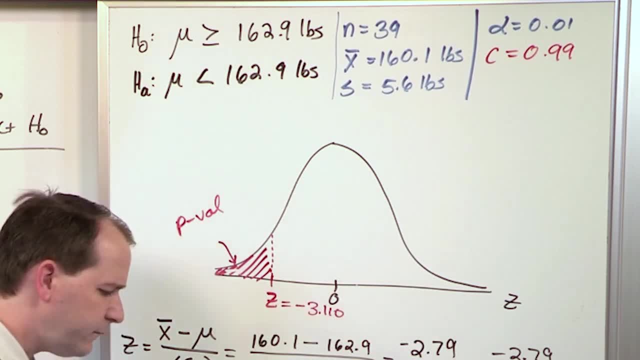 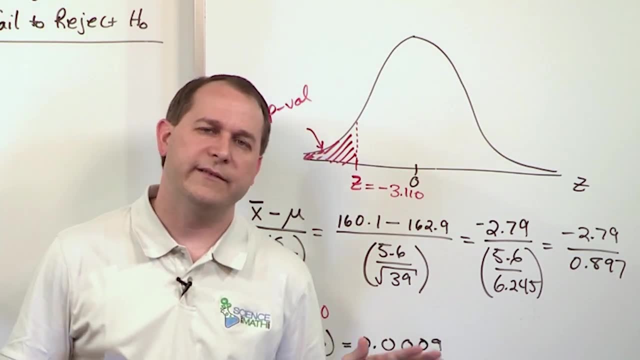 from our data would be falling inside of the rejection region. So I hope, from doing all of these problems and talking about it so much, That you can see that p-values. they are a little different way of looking at it And there is a reason why you see that used. 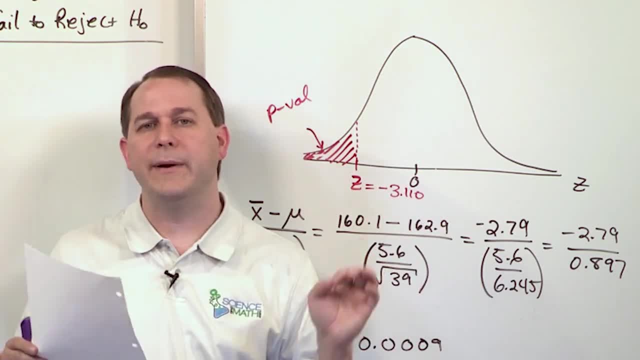 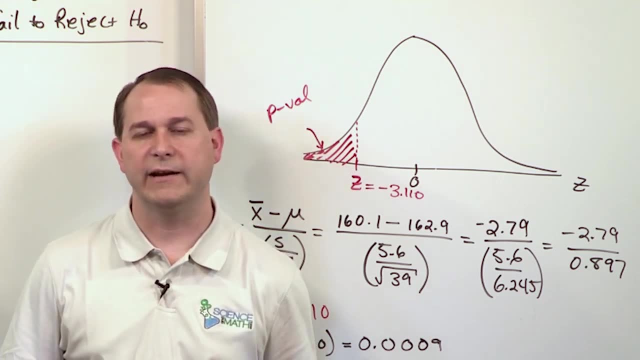 But in reality, especially for these kinds of problems, they're basically doing the same thing. You're basically getting a different way to look at the criteria that we use to reject the null hypothesis, And that's really all that they're for. So make sure you understand this in your journey through statistics. 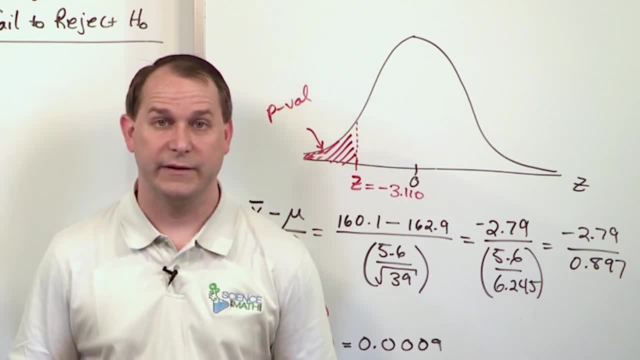 Solve this problem, Solve the other problems. We have lots more material to go in the sequence of courses. Following on to the next section, we'll continue to talk about the p-values. So if you're interested in learning more about the p-values, 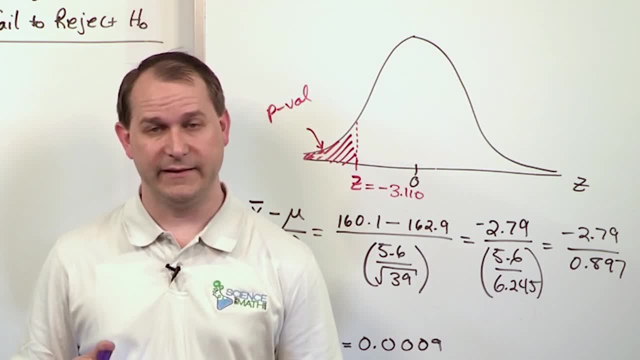 you can go to the p-values website at the bottom of the screen And if you're interested in learning more about the p-values, we'll continue working with hypothesis testing and statistics. Learn anything at mathandsciencecom.